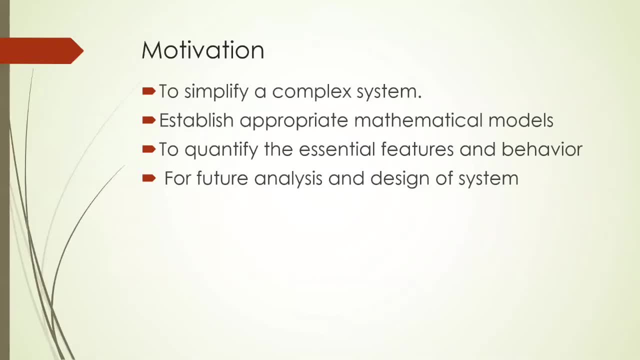 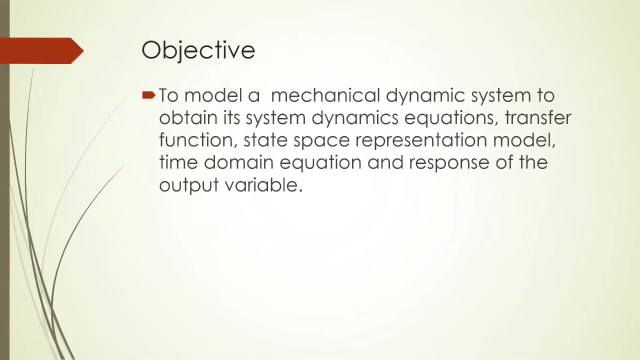 for the system, to quantify the essential features and behaviors of the system and provide help for future analysis. The objective is to model a mechanical dynamic system to obtain consistent dynamic equations: transfer function, state-space representation model, time domain equation and response of the output variable. 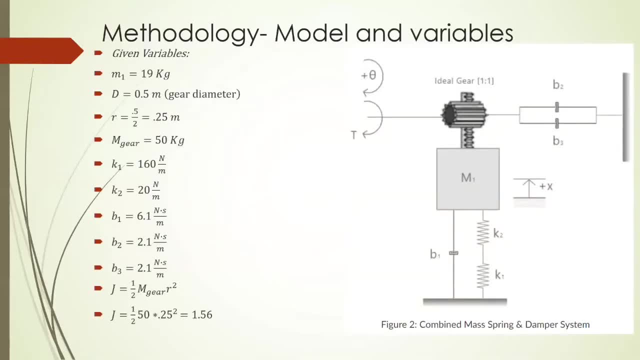 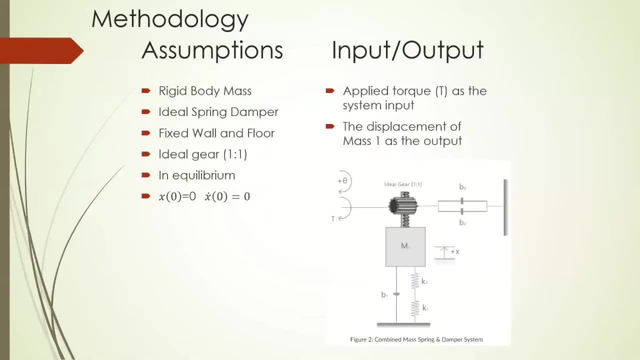 The system we will be modeling is a combined mass spring and damper system and these are its given variables. The assumptions for these systems are that it is a rigid body mass, has an ideal spring damper has a fixed wall and floor, has an ideal gear and is. 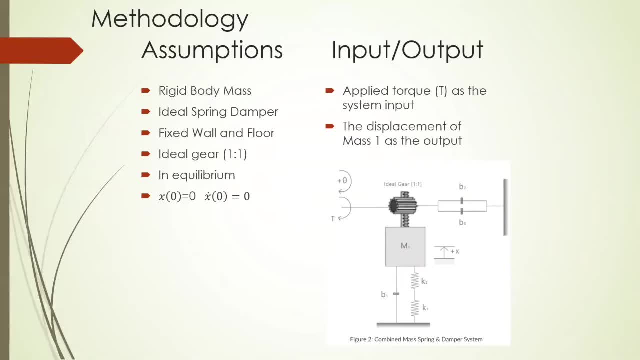 at equilibrium. within initial conditions equal to zero chili- or initial conditions equal to zero, input will be torque and output will be the displacement of mass. 1. The system has two main inertial elements: the mass and the gear. So out of those two elements we will make our 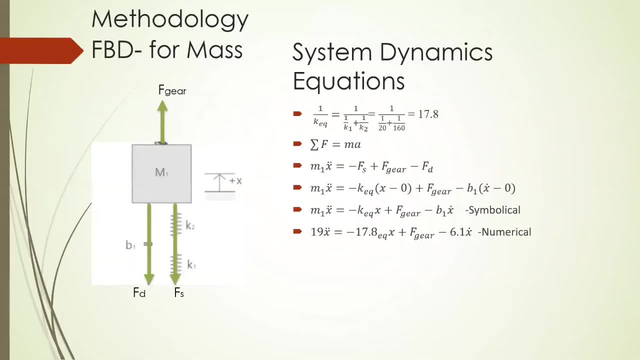 free-body diagrams. The free-body diagram of the mass will have 3 forces acting on the mass center, which we shall call free-body diagrams. This idea of the higher wind forces specific to the circon Teller-Maffet element is used as the guider in the geologic diagram For many different 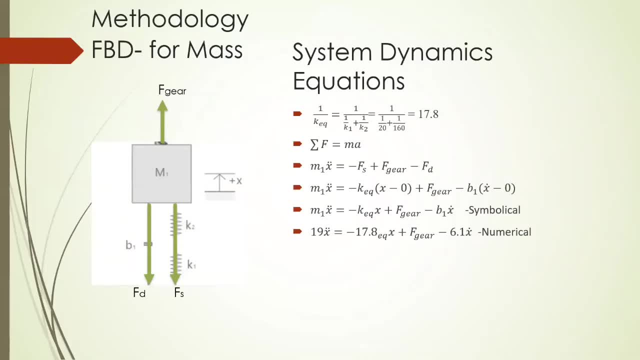 balloons, special evidential force pré žol int or incon sneaking of meters, will have to be applied as a bloom. The program should avoid the change in the analytical movementsero forces acting on it: the spring force, the damper force and the force created by the 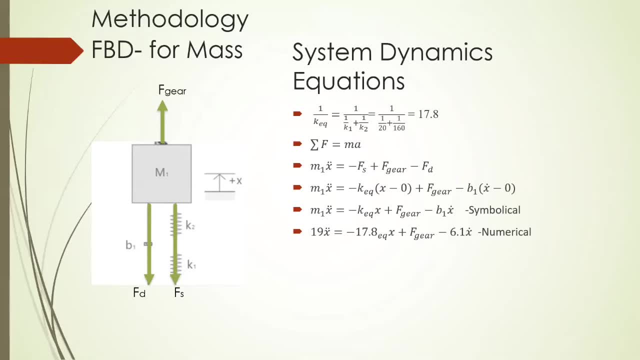 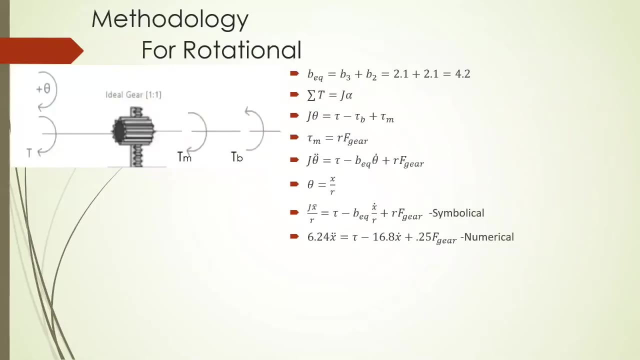 gear. First we will unite the spring and series to combine the spring forces And then, using Newton's law, we will set our dynamic equations where the summation of forces is equal to the acceleration of the mass. Then we analyze the gear that has a rotational motion. 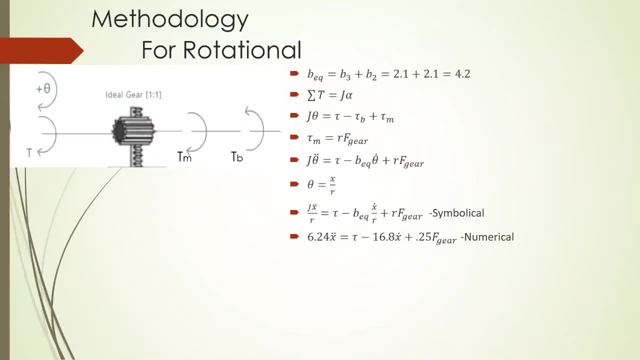 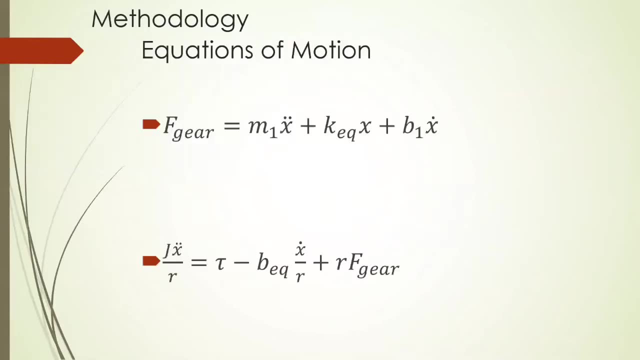 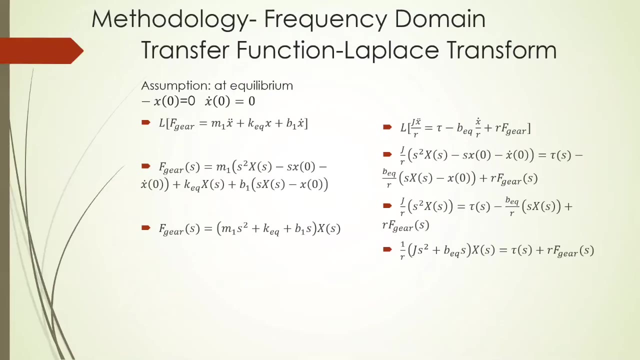 So Euler's law is applied to get our second dynamic equation. We also combine the dampers in parallel by adding them And we got our equations of motion. that will help us as we do frequency and time modeling First. we start with frequency domain modeling by applying Laplace transformation to both. 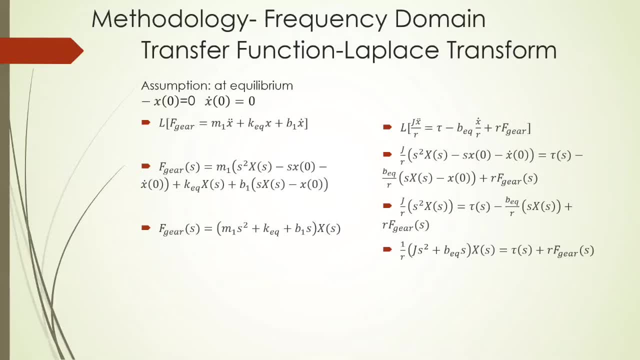 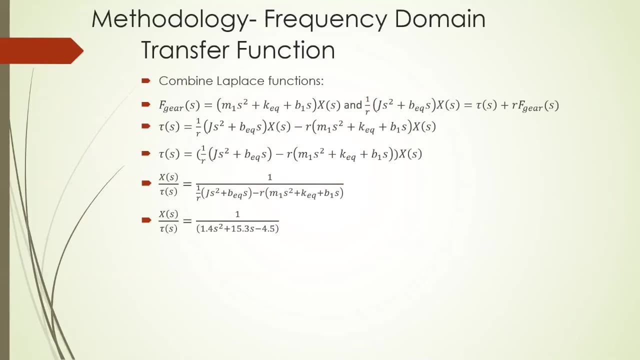 of our equations, The assumption that equilibrium comes in handy here because it simplifies the Laplace process by only leaving displacement as function of s and getting rid of the initial conditions. The Laplace equations are then combined to obtain the two equations, The transfer function having displacement of the mass as output and torque as input. 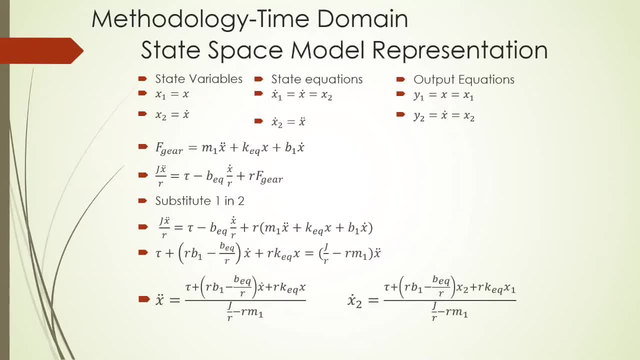 For time domain. the dynamics equations are brought back to create the state-space model representation. But first the state variables must be established. X1 will be displacement and X2 will be velocity. It will make our state variable X1 equals velocity. 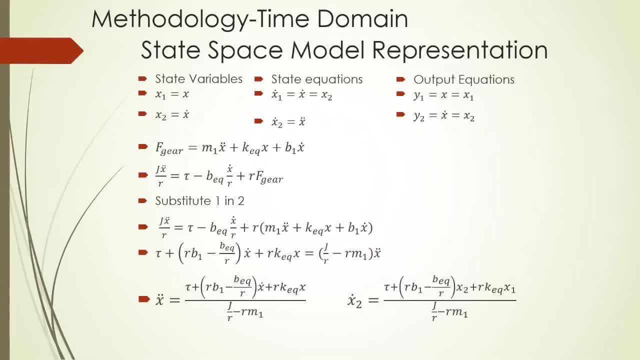 That is equal to X2, and our X2 state variable equal to acceleration. For output equations the common variable used is Y, So Y1 and Y2 will be used. Y1 will be set equal to X- that is, X1, and Y2 will be equal to X2.. 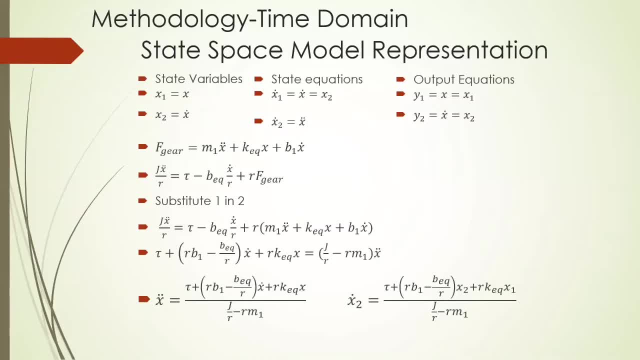 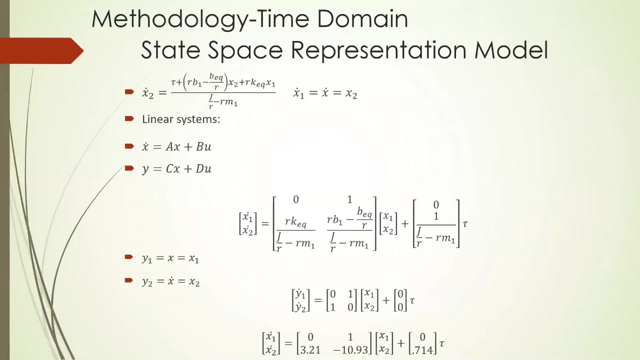 This is done in order to facilitate the state-space model equation. Acceleration is then isolated by combining the dynamic equations and the variables are replaced with state variables. For a linear system, the model is as follows. You can see: X equal to AX plus BU and Y equals CX plus U. 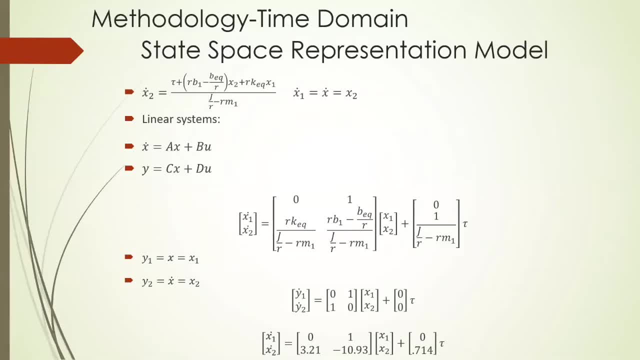 A, B, C and D are all matrices And, And here we set them up with x1 and x2 equal to that matrix, And you see that x1 is equal to x, dot equal to x2.. So there's gonna be a zero and a one. 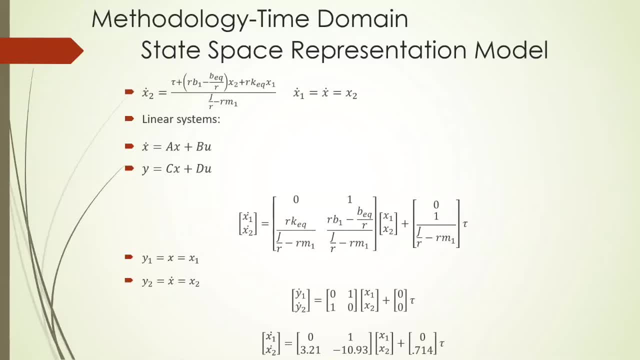 Now for x2, the state variable x2, we're gonna have that whole equation. So for the first, for x1, we have r times kq over j over r minus rm1.. And then we can continue with those and obtain this equation right here. 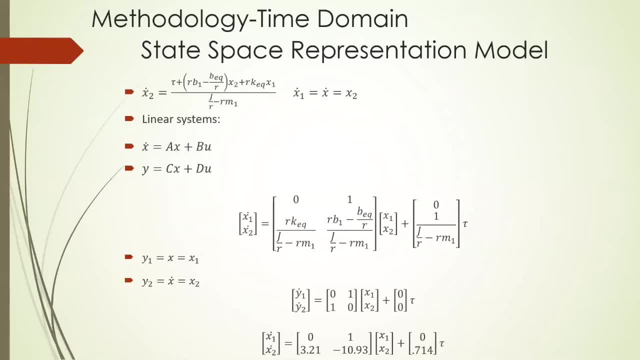 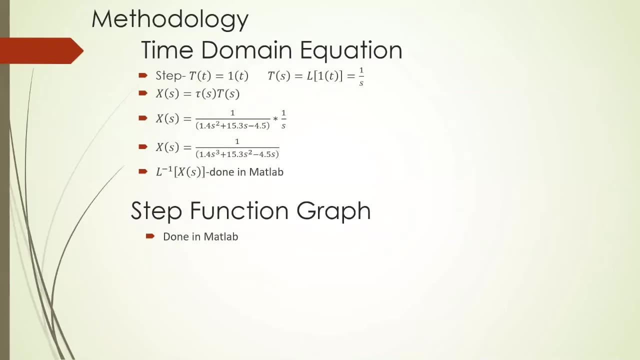 For the output variables, we have y1 equals x equals x1 and y2 equals x, dot equals x2.. And that gives us this matrices And we obtain the time donation equation, the time domain equation. In this case, it is a step response.